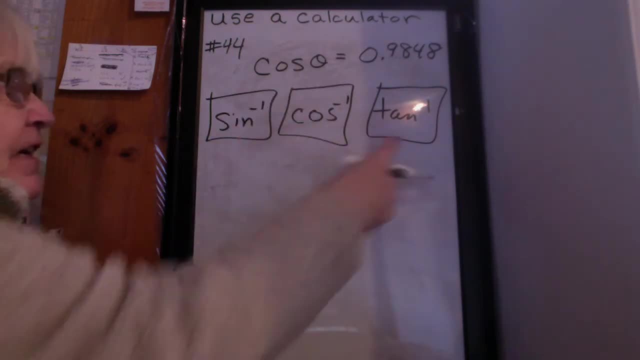 So which key do you think I'm going to use for this one if I want to find the angle, when I have the answer to the cosine of some angle, What is the angle? Again, that's cosine. so I'm going to use the cosine negative 1 key. 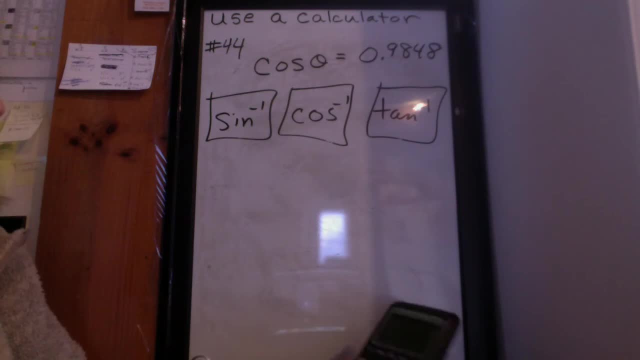 Now again, they asked for degrees. so make sure you're in degree mode And then it's pretty easy. You clear out your calculator and then you type in the cosine. You clear out your calculator and then you type in the cosine negative 1 key by using the yellow button first. okay, 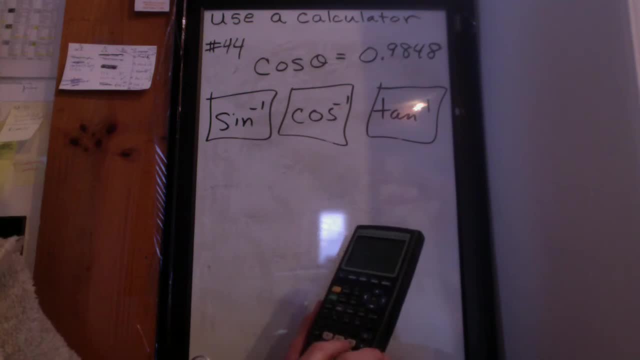 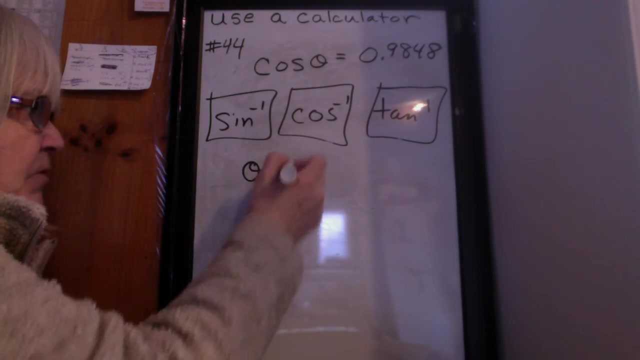 And then you're going to type in 0.9848, and then hit enter And it gives me 10.0025.. So that means that theta equals 10.0025 degrees. Now, if I asked you to round it to the nearest degree, 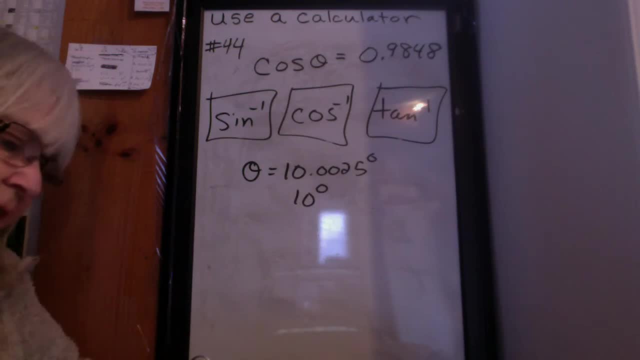 then you could say 10.0025 degrees. If I want the radians for that, I can change this to radian mode and do the same thing. So I'm going to hit my mode button and I'm going to change now to radian mode and hit clear again. 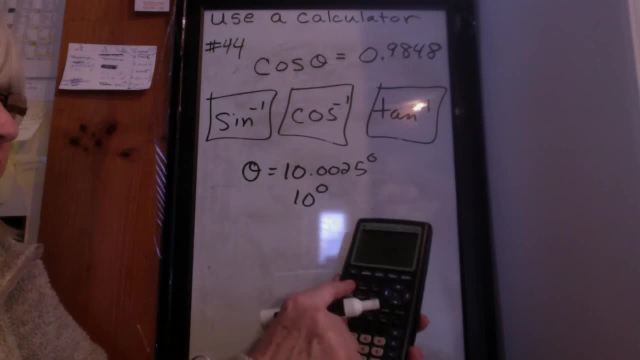 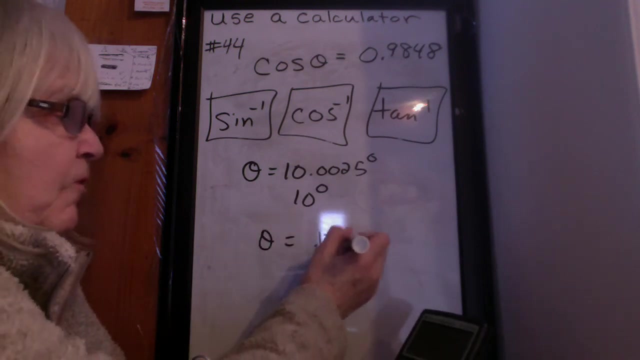 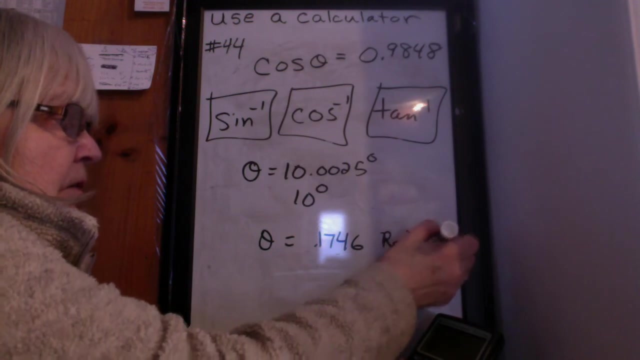 And now do again the cosine negative 1 key. so second cosine Type in 0.9848.. And this time my answer should be in radians, and theta equals 0.1746 radians. okay, So the calculator will figure radians or degrees for you. 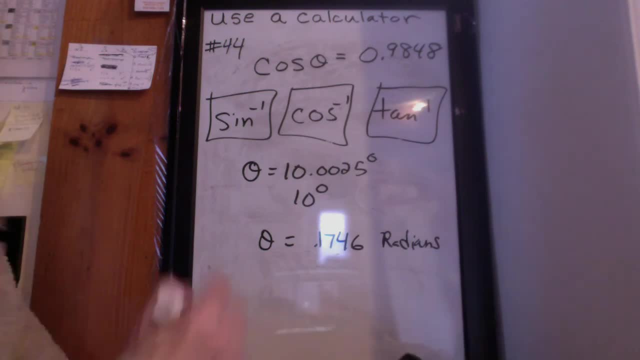 Make sure you're aware of what mode you're in and pay attention to what type of answer they want. Do they want degrees or radians? And then you're going to type in 0.9848.. And these are pretty straightforward. 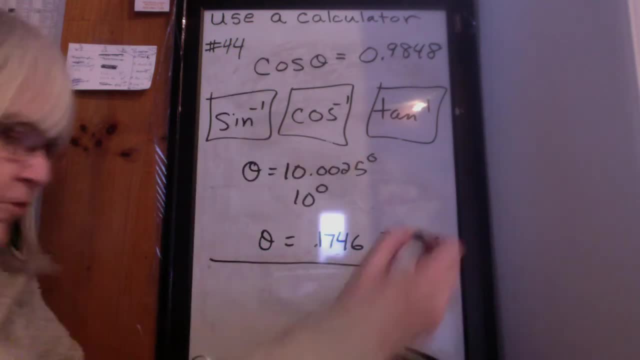 But what happens when I do some of the partner functions? For example, suppose I want to do cosecant of theta equals 3, right. There's no cosecant button, So the only thing I can do is the sine of theta right. 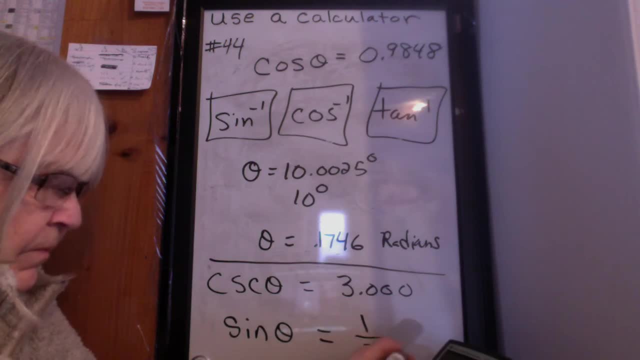 And use its reciprocal. So I use the sine inverse key, So second, And then I do, and I put this in parentheses. So parentheses 1 divided by 3.000, close parentheses, hit enter and I get the radians. 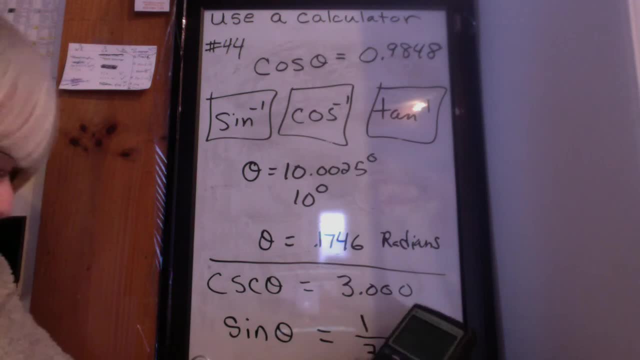 I get the degree in radians. and did I want radians? No, I didn't, I wanted degrees. Well, I didn't change my calculator, So it's 0.339.. 0.339 in radians. let's check it out in degrees. 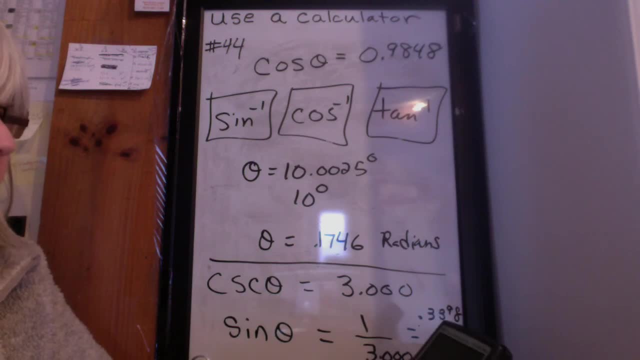 So let's change my mode. Let's go back to degrees. enter. all right, clear it out. So now I'm going to do the sine inverse of 1 divided by 3.000, and I get 19.47 degrees. 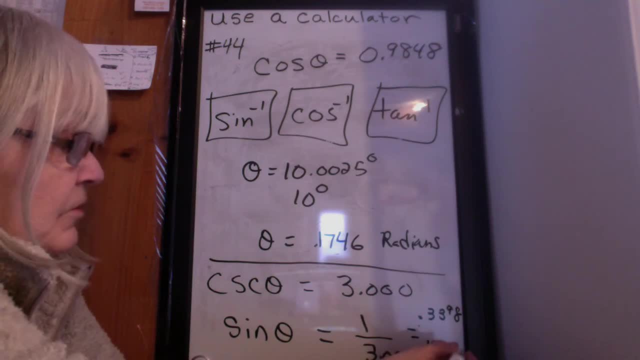 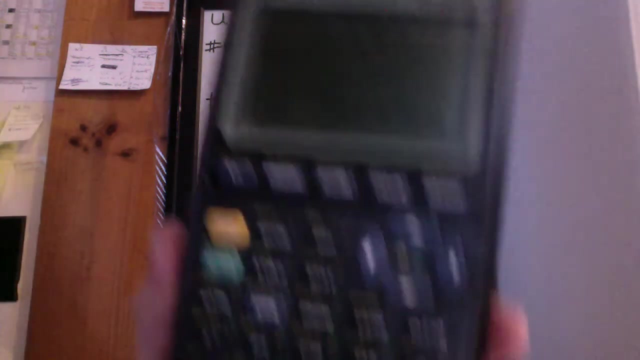 19.47 degrees, And you know I could check. I could change it to radians and see if I got the right radians. Do you remember the conversion Times? something by what? Pi over 180,? right? So times pi divided by 180, and I get 0.3398. 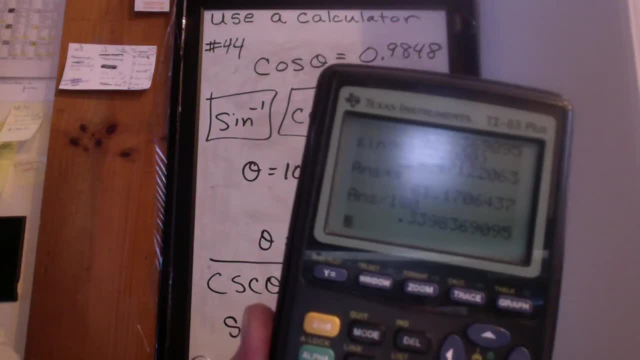 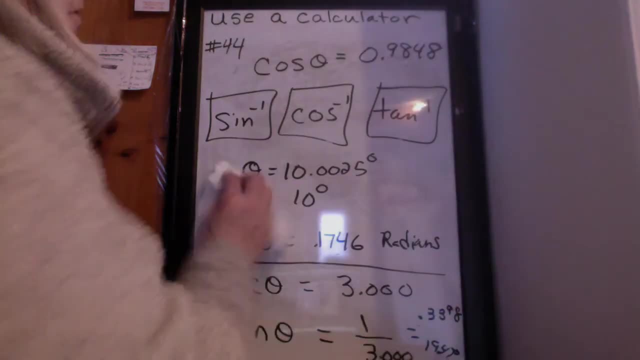 So I did the conversion. I'm going to check to see if I can figure out the radians by using my formula, but of course you can put this in radians also. So do we want to do one more of these tricky ones? 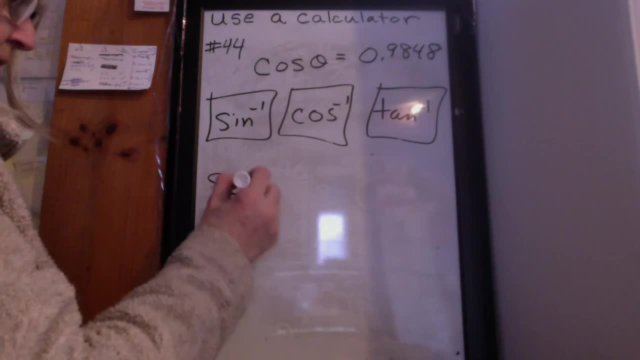 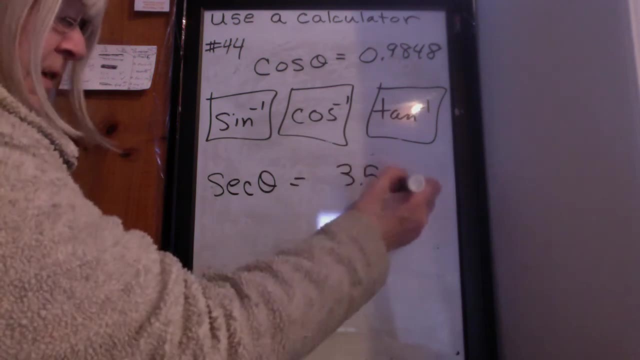 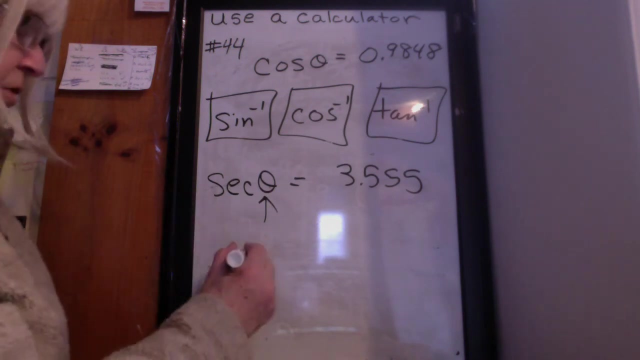 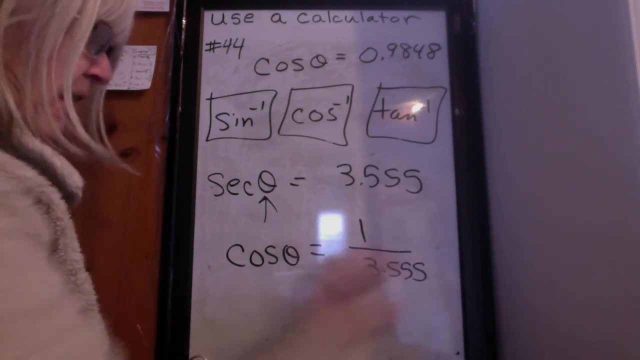 Let's try one more. So suppose I want the secant of theta equals 3.555, and I want to know what the theta is. Well, what's the partner function for secant Cosine, Cosine? So cosine of theta would equal 1 over 3.555.. 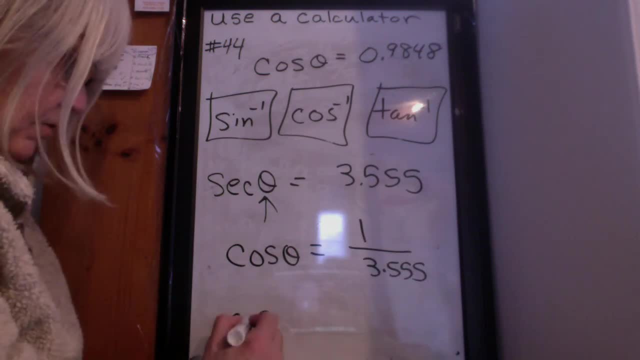 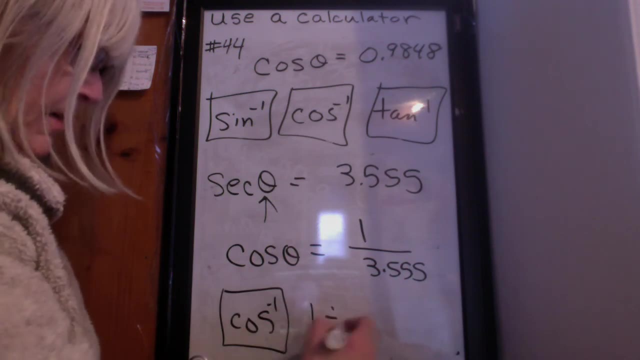 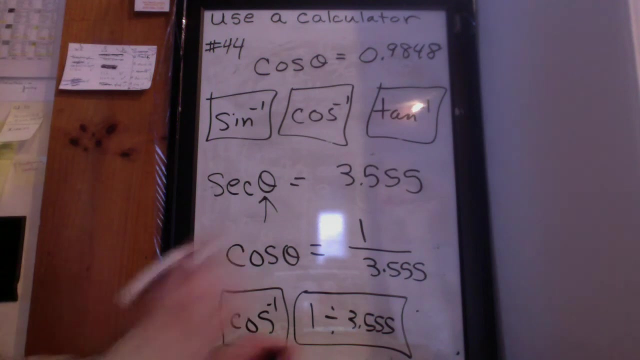 And then now use the cosine negative 1 key right And then type in 1 divided by 3.555, and then hit enter and you should get the answer. And the answer should come out to 73.7 degrees.